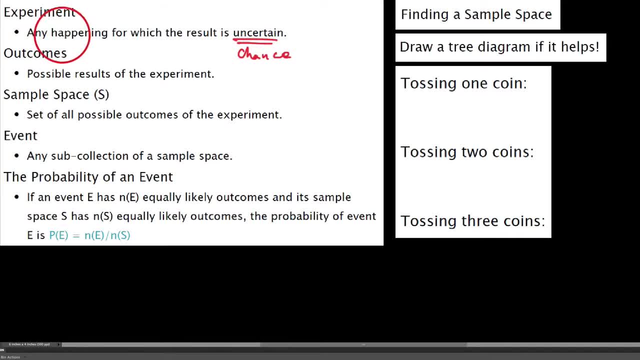 So outcomes, when we talk about the outcomes of an experiment, these are the things that are possibly going to happen, So it doesn't have to happen, but the set of all possible outcomes- that's something we're going to refer to very specially to- is our sample space. 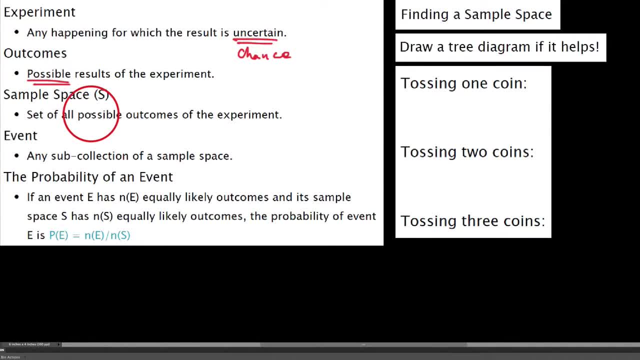 So when we take all the possible outcomes for an experiment, say like a coin, you know tails and heads, that set of all possible outcomes is what we refer to as the sample space, And that is kind of contrasted with the event space, which is any sub-collection of a sample space. 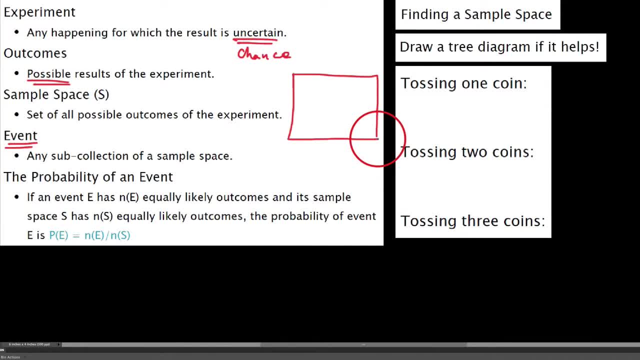 So what we're going to do here is just very, very quickly, we're going to illustrate what we mean. But this right here We represent the sample space. You know, if we look at this in like a Venn diagram sense. 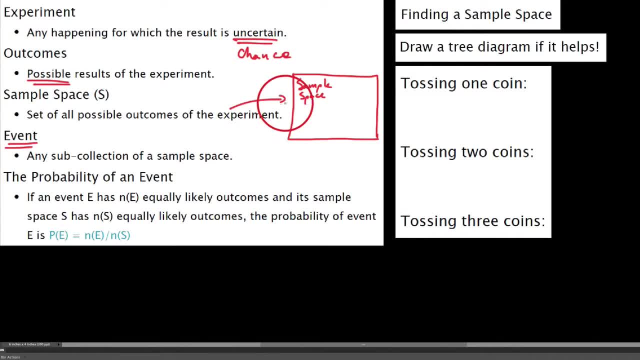 So the sample space is the set of all possible outcomes for an experiment. The event space is just a subset of all the possible outcomes that we're maybe interested in, And we could refer to this here as the event space, And I probably should have written it on the inside. 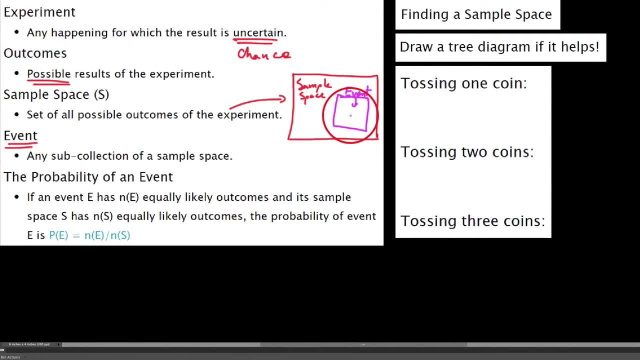 But you know, like, if you were to imagine rolling a die, the event that you roll an even, you know the two, the four and the six would be in this little even bubble, And then the one, three and five would be out here in the not even bubble. 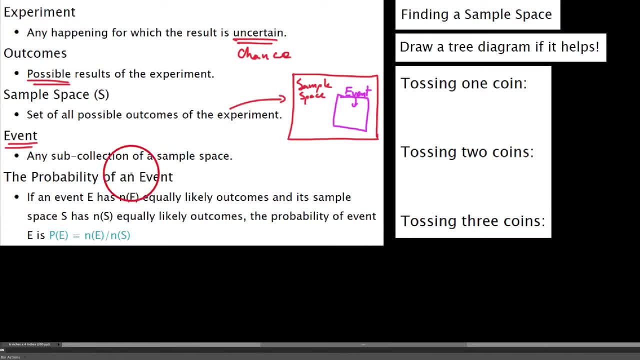 To account for all possible outcomes, one through six, So the probability of an event. Let's go ahead and get to the nitty gritty here. We basically say that if an event E has N of E, Now this N of E is basically- we're going to make a little note here. 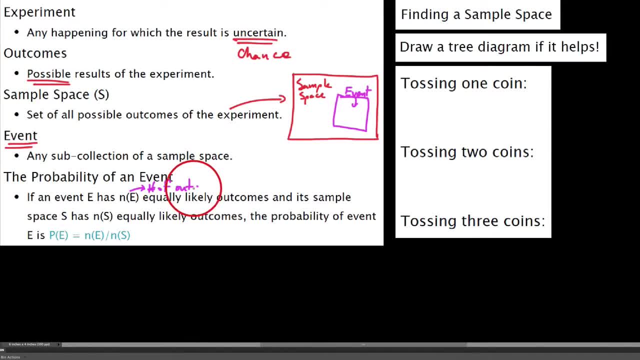 This is the number of outcomes in the sample- or sorry, not the sample space, the event space. So essentially, the number of possible things that give us this particular event in its sample, in our sample space here. Basically, let's read through this here: 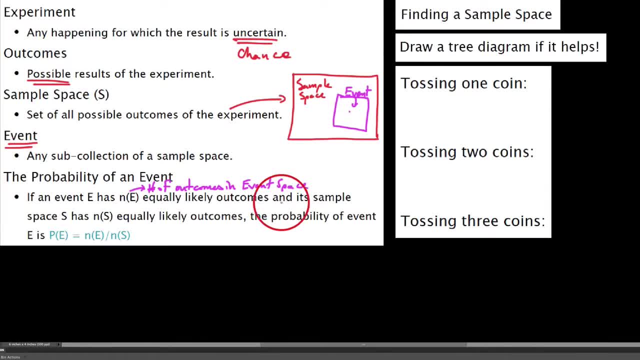 It says if an event E has this many equally likely outcomes and its sample space S has this many equally likely outcomes, And the probability of an event E occurring is P of E, So we're going to read this as the probability probability of E occurring. 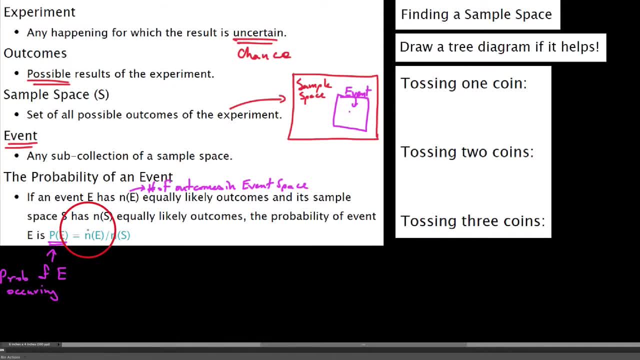 We never read the occurring part, But basically the probability of E is equal to the number of ways we could get this in the event space divided by the total number of outcomes- here The number of things in the total sample. So for instance, if we were to say the probability of rolling a two on a die, we would say that really it's just six total outcomes. 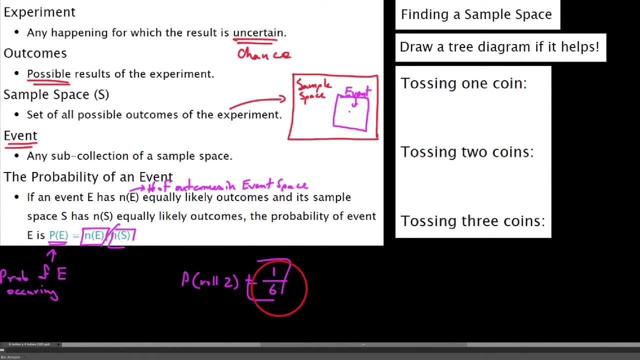 One of them gives us a two in that event space, And so the probability is one out of six. So, before we get into anything special, what we're going to do is practice finding a sample space. It's going to be imperative to what we need to do. 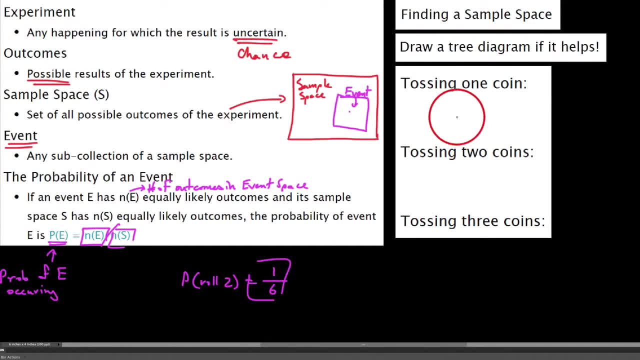 So I notice here it says: draw a tree diagram. if it helps, Let's do this To find the sample space or the set of all possible outcomes. we usually write this as a set of things here, And so when we say, tossing a coin, what's the set of all possible outcomes that could happen? 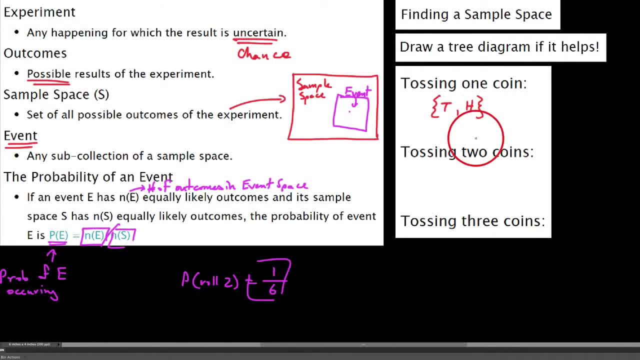 Let's say that it's either going to be a tails or it's going to be a heads, or a heads and a tails. You can listen either way, But this is the sample space for this particular experiment of tossing one coin. Now, the moment we toss two coins, the interesting thing happens is we could either have like a tails and a tails, or we could have a heads and a heads. 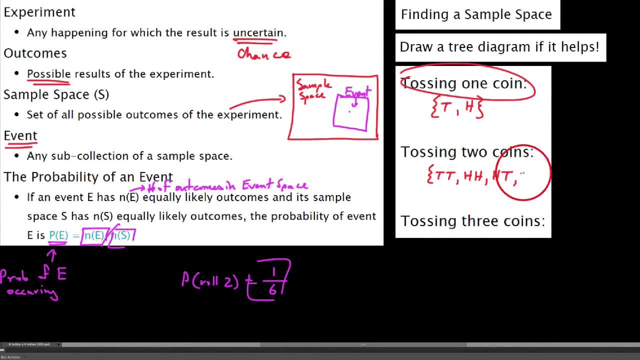 And also we have to account for the fact we could get a heads on the first coin and tails on the second one, or tails on the first one and heads on the second one, But this would be the set of all possible outcomes. You can see that it's four times as many as what we started with. 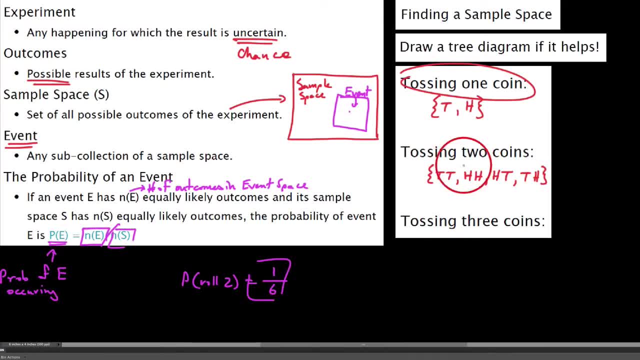 Now the interesting thing here is when we toss three coins. this is where the tree adapts. The diagram might come in handy. So what we're going to do is we're going to kind of draw like an original point over here on the left. 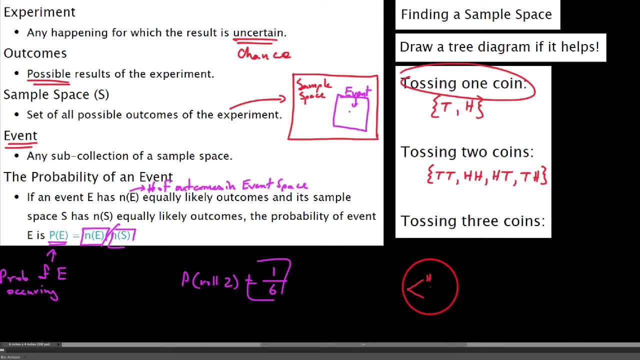 And we say that for our first experiment, the two outcomes, we'll list them here. We say either heads or tails, And so at this point we would say: well, if we were to flip now a second coin, what are its possible outcomes? 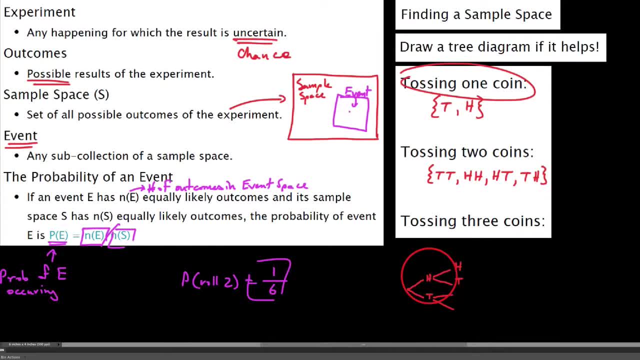 And its possible outcomes. from heads could either be heads or tails. We get a heads and a heads, or a heads and a tails, Or we get a tails and then a heads, or a tails and then a tails. These are the possible outcomes. So out of these here we're going to get more branches that pop out of this. 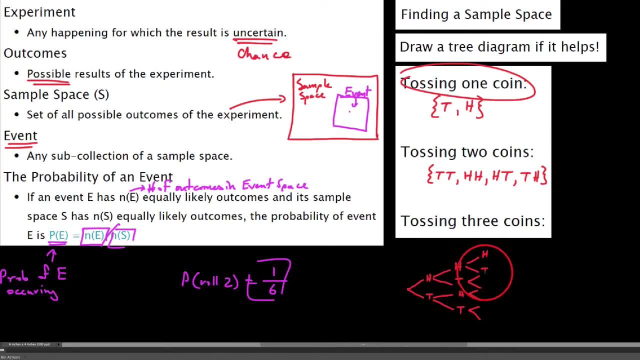 And essentially we could see that We get a heads heads heads or a heads heads tails, A heads tails heads or a heads tails tails, A tails heads heads, A tails heads tails. 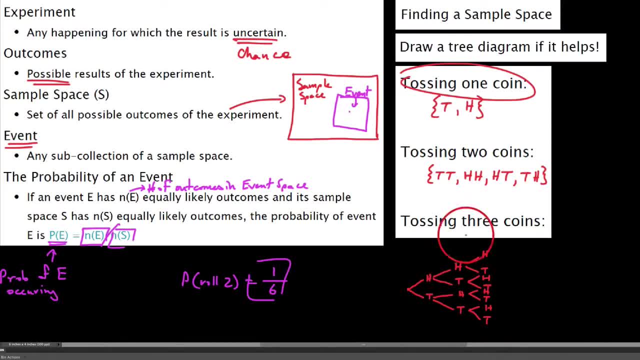 Or a tails tails heads and a tails tails, tails. So we can see that tossing three coins here we would have eight possible outcomes. Excuse me, If we could list them all, we could say: heads, heads, heads. 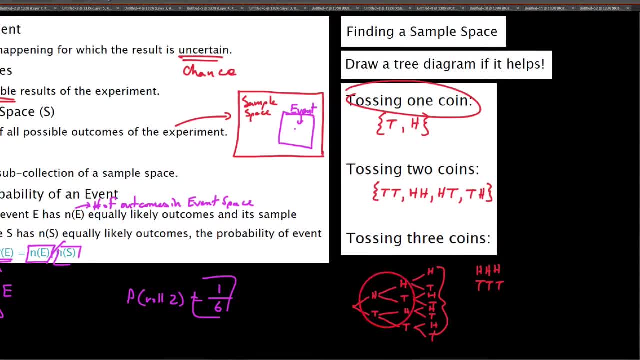 Heads, heads, heads, Tails, tails, tails. Those were listed on the outside. here We could say heads, Heads, tails. We could have a tails tails heads. How about a heads tails, heads, Tails, heads, tails? 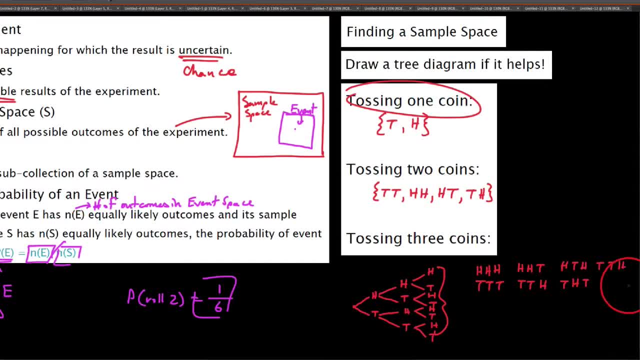 And then a tails tails heads And a heads tails, tails, Heads, heads, tails. Pardon me, So here are the possible eight outcomes here, And we should separate these with commas, And I didn't, I'm sorry. 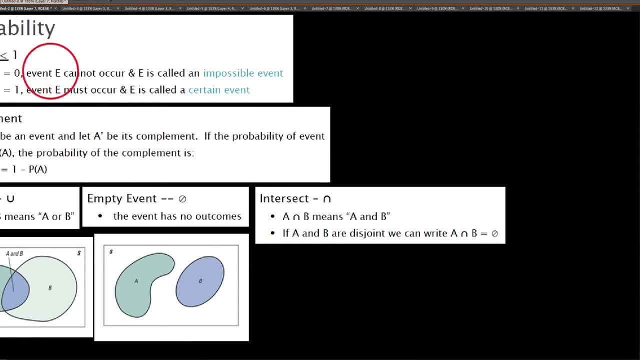 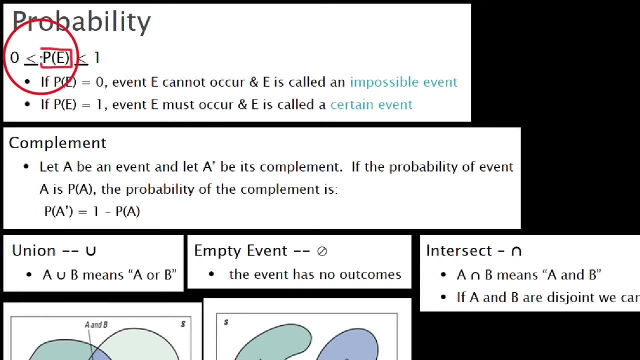 But basically the sample space is the set of all possible outcomes for an experiment. So let's go ahead and get into the probability here, symbolically. First thing we want to notice here is this: P represents the probability that something actually happens, And the first thing we're saying here is that a probability can be zero. 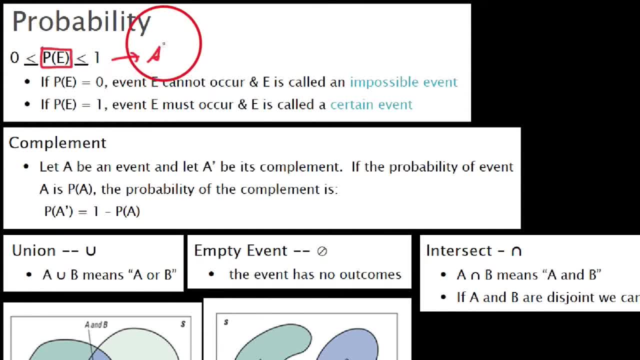 It can be one, But it's between zero and one, And so we'd say there's always a number between zero and one, Always between zero and one, and including zero and one. So when we look at things like the probability of an event occurring and we get zero for an answer, 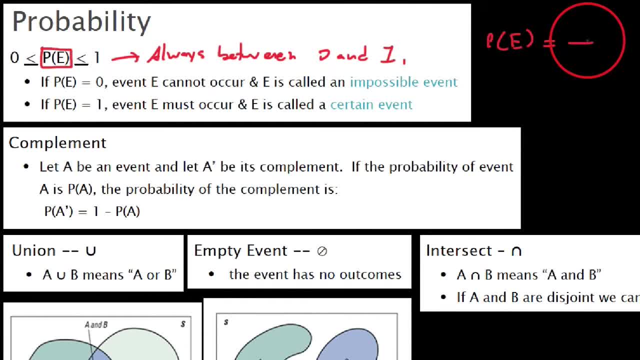 the interesting thing is we'd say, well then, the probability of the event occurring was there were zero possible things in the event space over whatever the sample space was, And that's what the size of the sample space is. But basically, since nothing gives us that particular event right there, what we get is just a big fat zero. 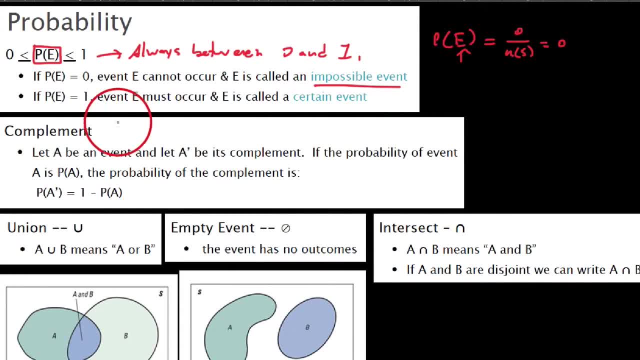 So, if nothing gives us this- we're going to refer to the probability of an event being zero as an impossible event, and the probability of an event being one which is the same as 1.00, which is the same as 100 percent- then what we would see here is this: 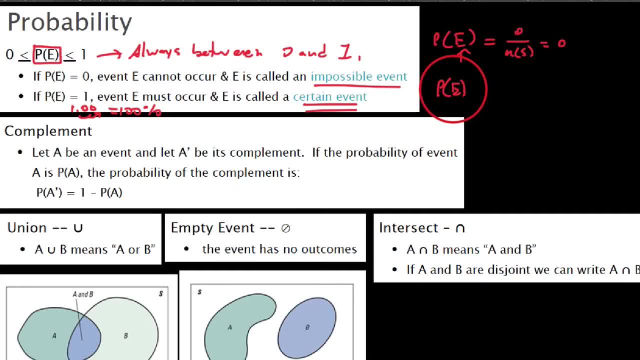 This is what we would refer to as a certain event. That would be something like if I were to write the probability of an event. an event, that's an either. you know, if I had something like rolling a die and say one or bigger, you know well, all of them are one or bigger out of six possible. we'd say one or 1.00, or a 100 percent chance. 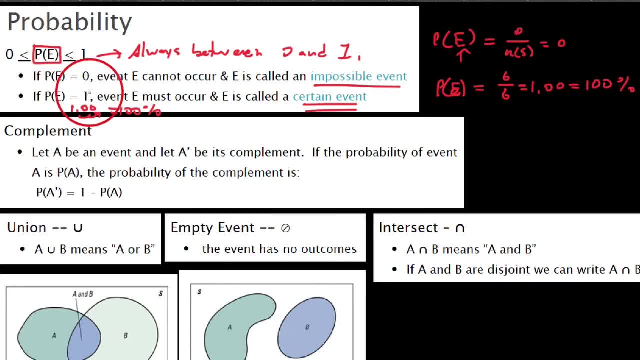 But basically impossible, and certain events have probabilities of zero. one and everything else in between is just some percentage. So let's touch on the idea of a complementary event. We say, letting A be an event and A prime is how we would read this here- A prime be its complement. 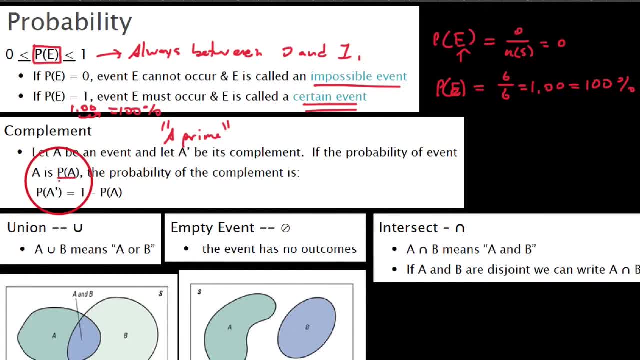 Basically we say: if the probability of an event is P of A, the probability of that event A, then the probability of it- excuse me, its complement- is the probability of A prime, and that's equal to one minus the probability of A. 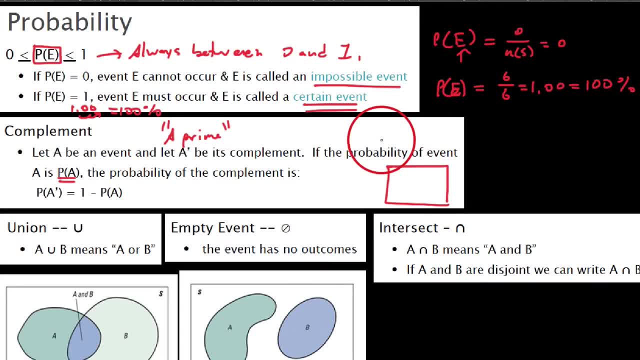 So what I basically want to do here is: I want to illustrate this. What we're saying is, if this is our entire sample space, right here the sample space, what we have is some event in here. we're going to call this A. 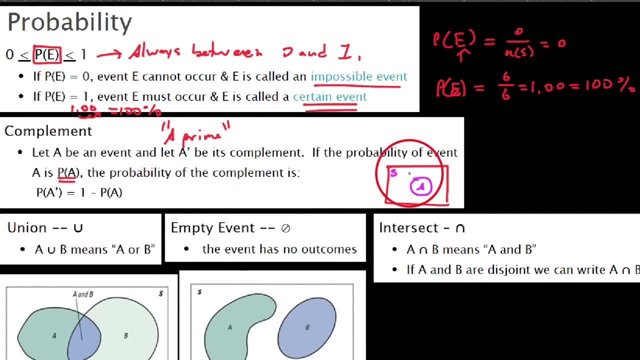 Everything that is not on the inside of A is what we call the complement of A And the definition of A prime. we could say: if A is this, then this can be read as not A, And that's what the complement of A means. 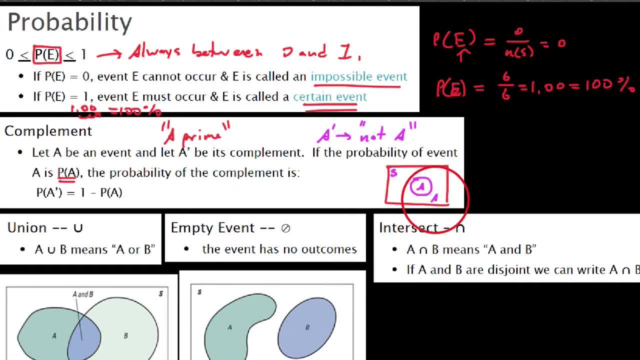 And so we would say: everything on the outside of A, within our sample space, is A prime. And so the interesting thing here is we have this relationship where, if we take the probability of A, which is just this part here, and we add it to the probability of its complement, 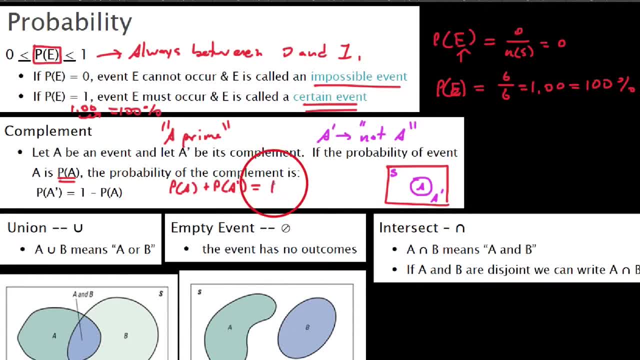 which is the probability of everything else but it. what we get is we just get the probability of the sample space, or, in other words, we just get 1.00 or 100%. So, with that being said, what we could say is: well then, if we want to find the probability, 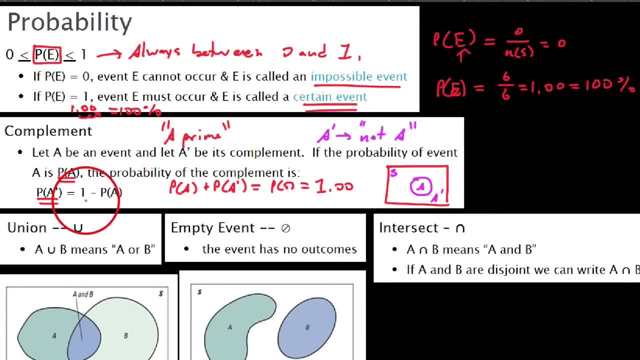 that something does not happen doesn't happen, then what we'll do is we'll take 100% of our stuff here and we'll subtract off the probability that it does happen, and what you get left with is all this stuff out here where we have the probability of A complement. 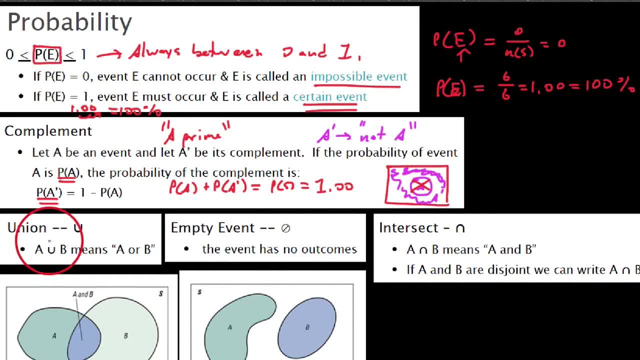 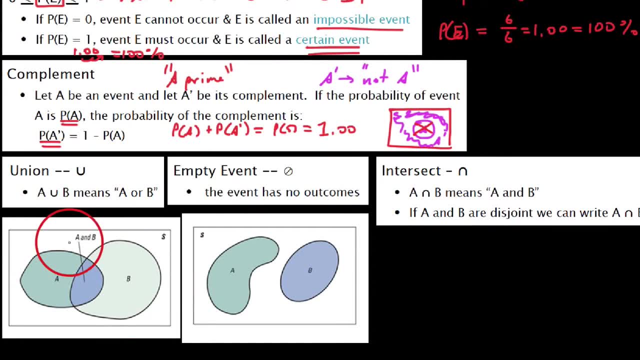 which is just the whole thing, minus the probability that it does happen. So really quickly here let's talk about unions and intersections. So what you see down here is this kind of Venn diagram representation. In either instance, you're going to see that this S represents the entire set of possible outcomes. 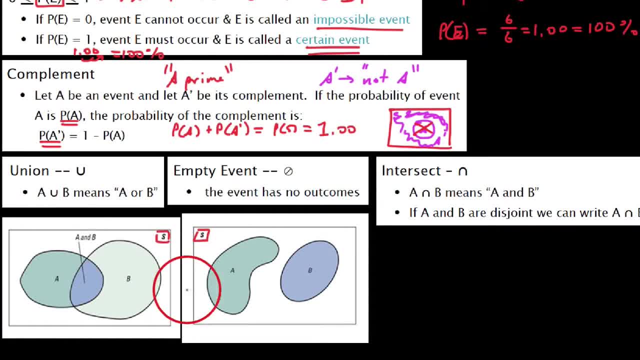 the sample space. So we have two events here, A and B, and under this first one here we're going to write a little note, here we say not mutually exclusive, And underneath this next one here we're going to write are mutually exclusive. 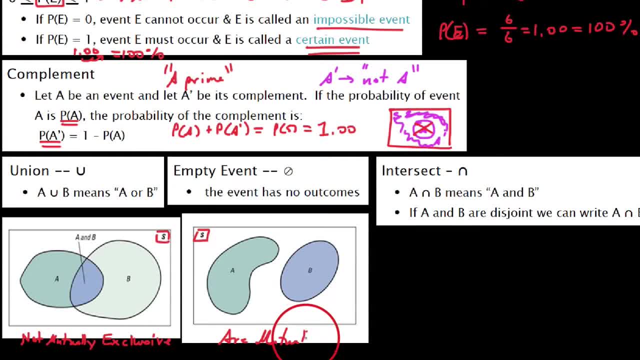 So we say are mutually exclusive. Now, when you exclude something, you leave it out. Mutual means between two things, like a mutual friend or something. So basically, mutually exclusive means that between one another they have nothing in common. There's a big fat gap between them. 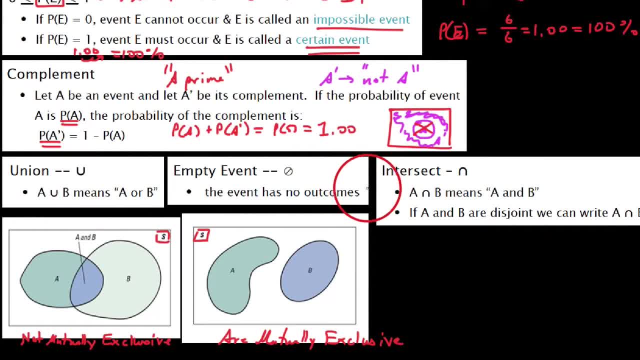 These are not mutually exclusive because they share things in common. So, with respect to unions and intersections, let's start with a union. We say that A union B, and this is how we write this. we would read it as A union B. 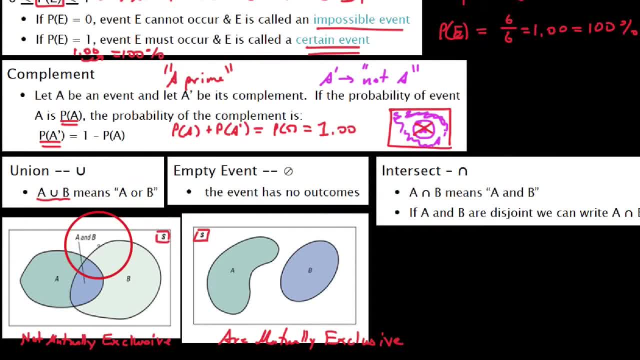 basically means that something can be in A or it can be in B, And so to represent A union B, it'd be either anything in A or B. it could be in either of these things within the sample space And likewise over here: A or B.